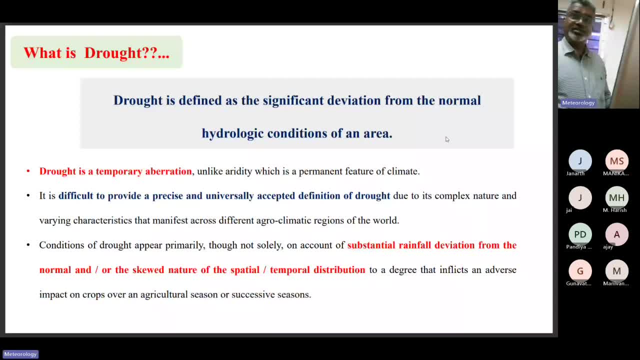 defined as the significant deviation from the normal hydrological conditions of an area, And drought is a temporary aberration, unlike aridity, which is a long term and a permanent feature of the climate. So drought is a temporary aberrations during an hydrological cycle happening. 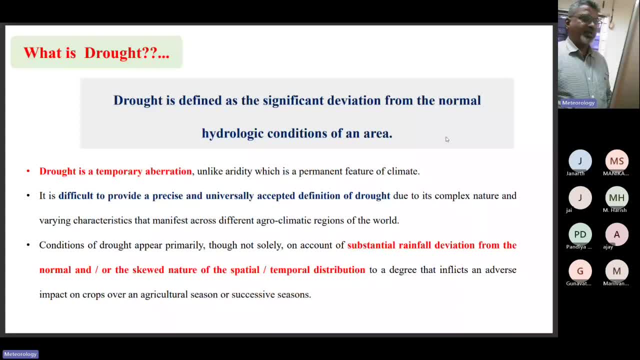 in a particular area, And it is difficult to provide a precise and universally accepted definition of a drought, due to its complex nature and varying characteristics that manifest across different agro-climatic regions of the world. The conditions of drought appear primarily through not only on the front of substantial 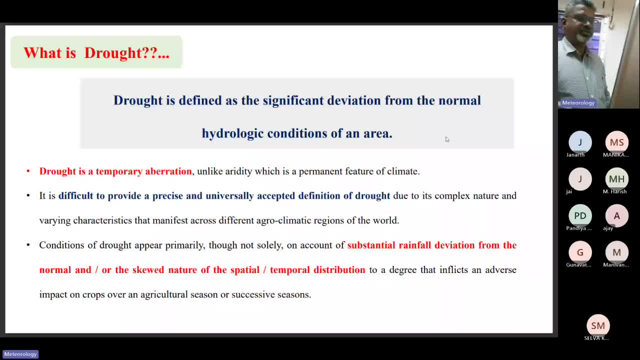 rainfall. deviation from the normal or the skewed nature of spatial or temporal distribution to a degree that inflicts the adverse impact on crops over an agricultural season or successive seasons. So coming to the classification of drought. drought is pursued by various people in different areas of the world. 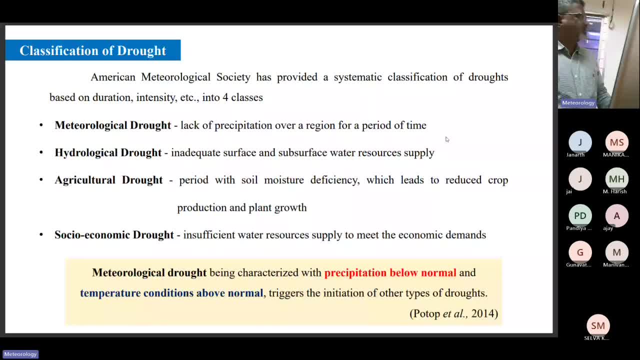 So the definition of drought will also vary. So American Meteorological Society has provided a systematic classification of droughts, based upon the duration intensity, into four classes. All of you may be knowing what is meteorological drought. It is nothing but a lack of reputation. 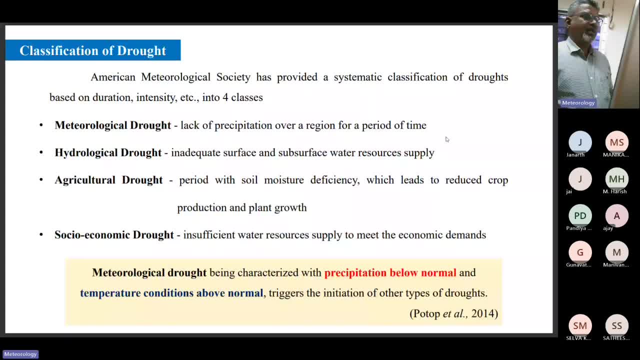 over a region for a significant period of time. Hydrological drought is an inadequate surface or the water supply or water resources, maybe in the dams, And agriculture drought refers to the soil, moisture deficiency and the road zone actually, which leads to reduction in the crop production and the plant growth. 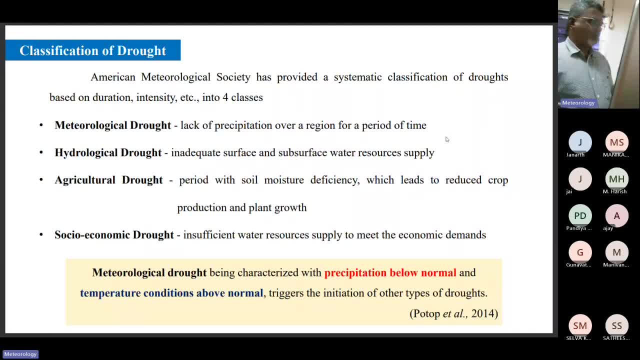 Coming to the socio-economic drought. the impact of all these meteorological, hydrological and agriculture drought resides in the insufficient water resources that are with the economic demands of the people living in the society. That is called the soil moisture deficiency, So it is an inadequate surface, or the water resources that are with the economic demands. 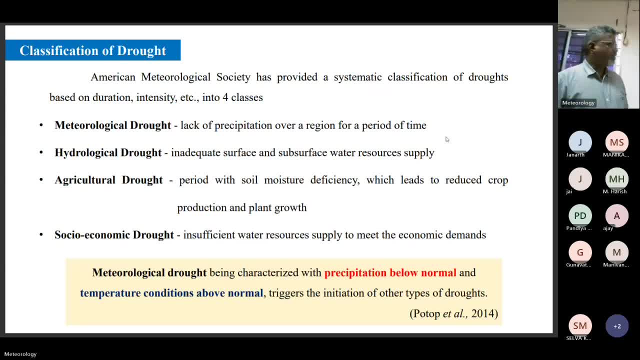 of the people living in the society, And then the impact of the soil moisture deficiency as a socio-economic threat. But we will mostly discussing, or limiting our discussions, on the meteorological doubt that is with respect to precipitation below normal or some temperature conditions above normal. These two trigger, all of you may be knowing, or very well was with this. figure: percentage departure of rainfall from normal for a country as a whole. that is southwest monsoon During successive drought years- you can see 1965-1966 and from 1999, there are consecutive droughts of 4 years, and last year also this year, we experienced a severe drought in Karnataka also. 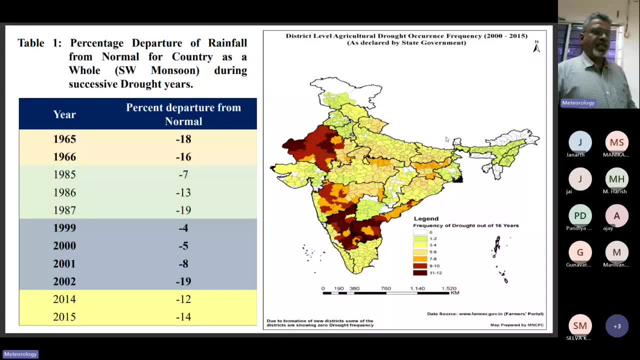 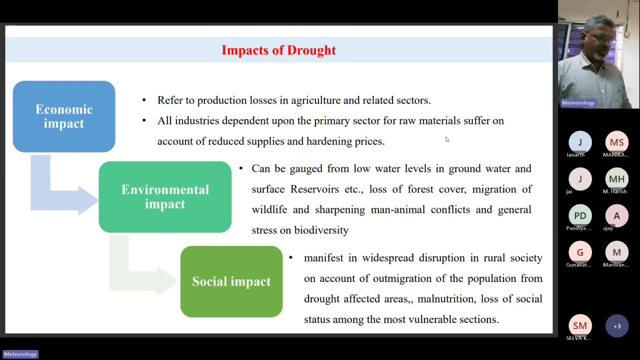 So most of the Rajasthana, parts of Maharashtra and most of the areas of Karnataka and Andhra Plains and Telangana very frequently experiences a drought compared to other states in India. Coming to the impact of drought, it can be classified into economic impact, environmental impact and social impact. 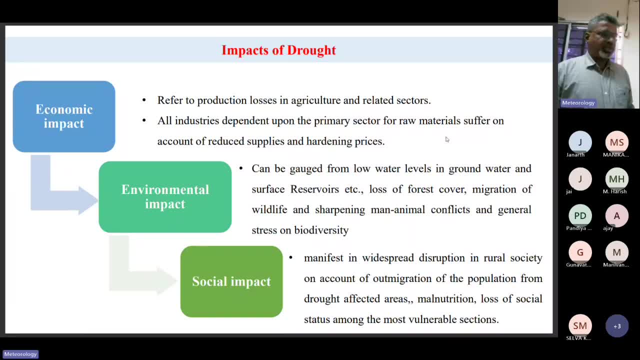 Coming to the economic impact, it refers to the production losses in, especially in agriculture and related sectors. because most of the industries depend on agriculture, those growth, as well as the production, is also influenced by the production in the agriculture. that is an economic impact. 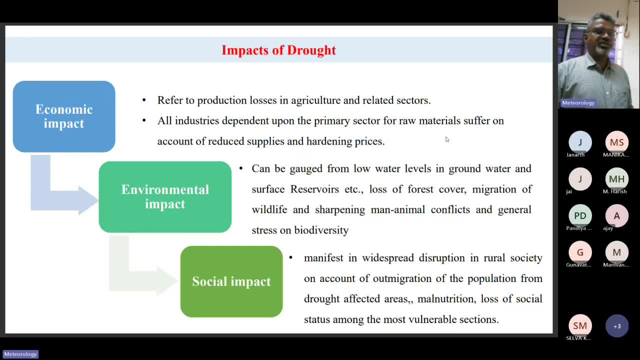 Coming to. the environmental impact can be gazed from the lower water levels in the groundwater or surface reservoirs, loss of forest cover, migration of wildlife and sharpening of the man-animal conflict that we are seeing very frequently. And another one is social impact. The economic impact and the environmental impact can put 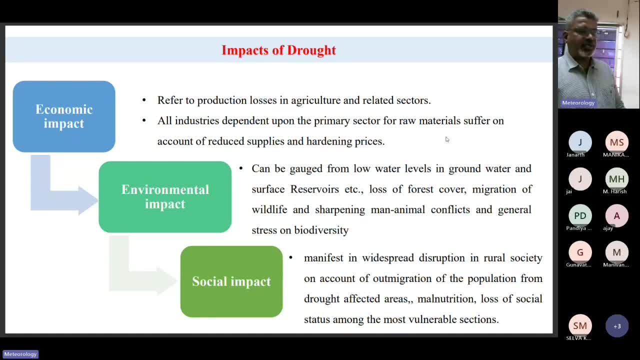 together and make a social impact. That is a widespread description of the rural societies and their economy, as well as the movement of the people from one place to other places. These are the two. So the response why we need to monitor this drought: Drought is going to occur. 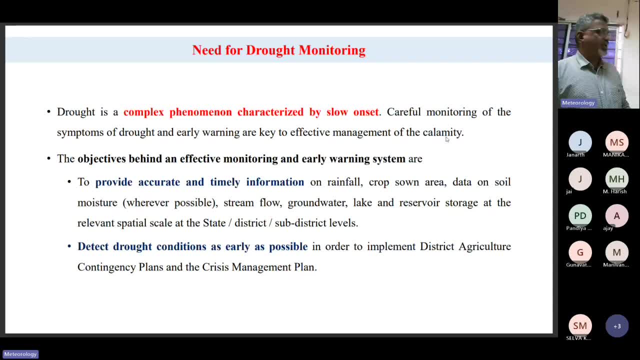 then why we need to monitor. So the response: why we need to monitor this drought: Drought is going to occur, then why we need to monitor? Because drought is a very complex phenomena and characterized by the slow onset that is creeping in nature. Drought it cannot come like the floods or like hurricanes or something. 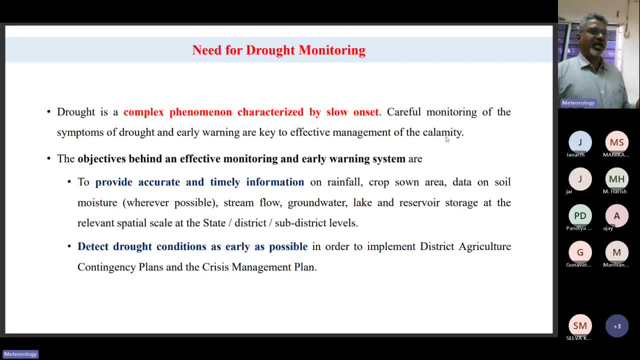 like that Occurrence of drought itself is a very slow process and we can see the manifestation of a few months or few years. That is why monitoring of the drought itself is very, very important, because monitoring the drought will tell us some warning signals that can be developed at the 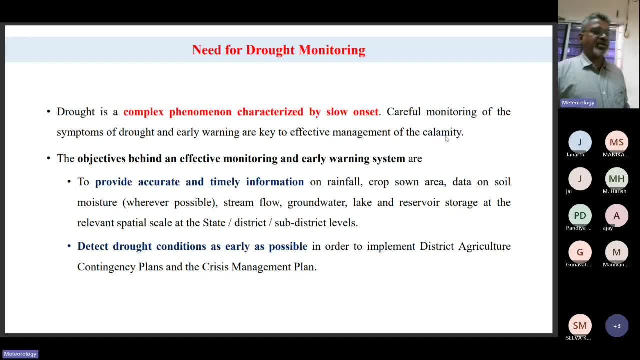 farming community. The objective behind effective monitoring and early warm system involves, first, to provide an accurate and timely information on the rainfall crops, one area, data on soil moisture and all. Second one is detection of the drought conditions as early as possible. If we detect the drought, its occurrence as early as possible, we can develop. 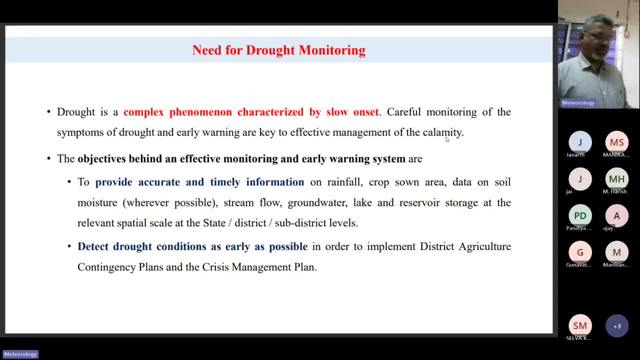 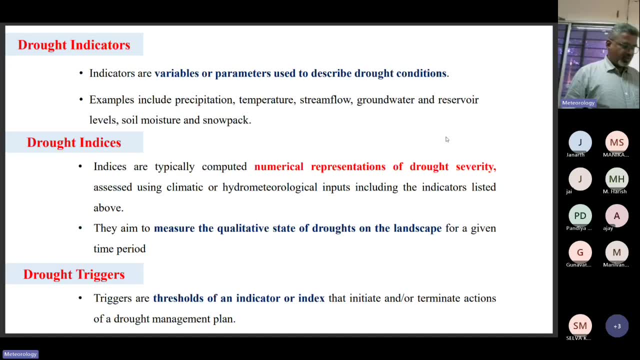 some contingency plans to mitigate or reduce the ill effects of the drought. For that purpose, monitoring of the drought plays a very important role. So drought can be monitored by various indices or indicators, or indices, and drought triggers. These are the three points from which the drought can be. 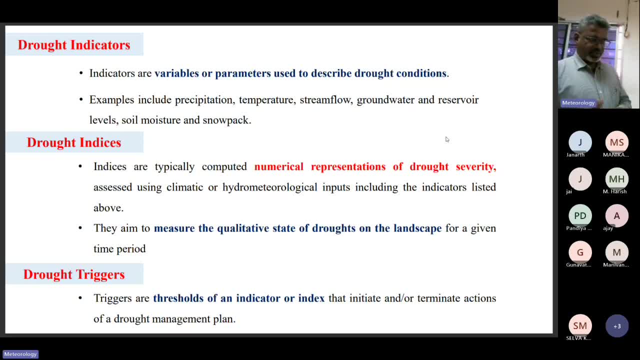 triggered or drought can be monitored, or drought indicators can be used for occurrence of the drought. Drought indicators Indicators are variables or parameters. Those are used for describing the drought. Examples: precipitation, temperature stream flow, ground water reservoir levels, soil moisture and snow peak. 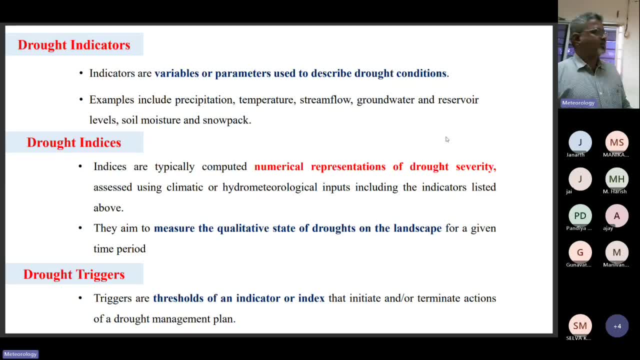 So these are the some of the parameters which we can measure. based upon the deviations to normal, we can say whether the drought is going to occur or not. there is an indicator. Indices means we are going to actually calculate by using the above measured parameters. 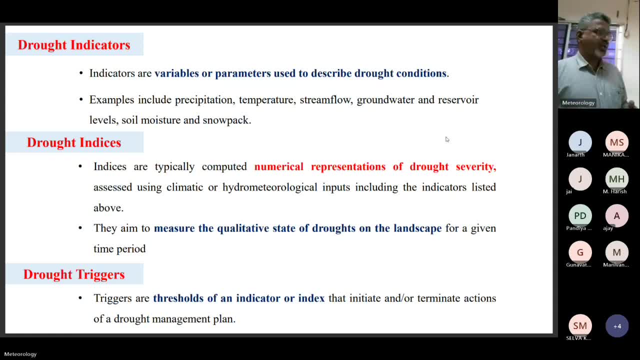 These are called numerical representation of the drought severity. Depending upon the value of a drought index, we can say whether the drought is large or medium, or strong or severe drought. and all these things And these indices mainly aims at measuring the qualitative state of the droughts on the 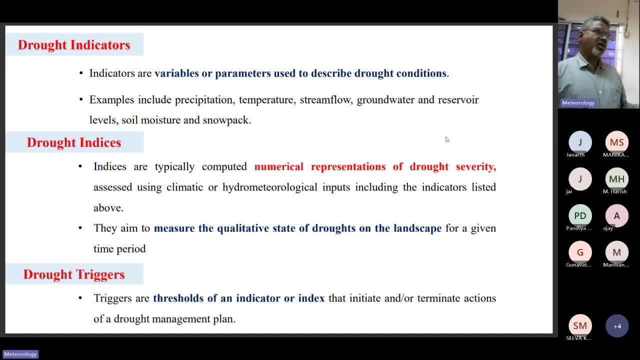 landscape over a large period of area, or maybe a taloka, or maybe a small area like a village, and all these things Drought triggers. that means to say these are the thresholds of indicators or an index. It clearly indicates whether the drought is triggered or not. 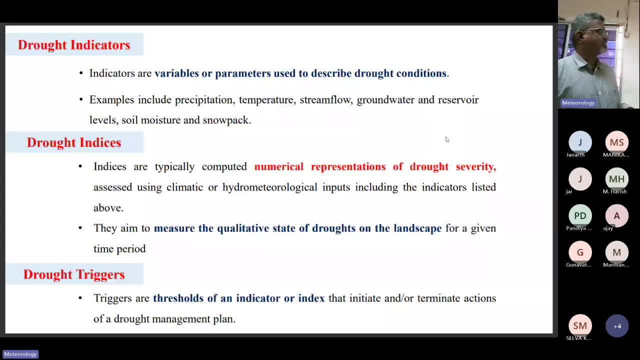 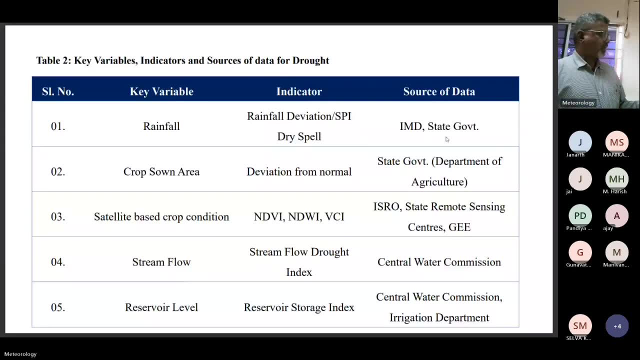 So these are the three differences between indicators, indices and the triggers. Coming to the key variables, one can be used for developing these drought triggers or drought indicators. One is the very well used parameter is the rainfall, So you can calculate a deficient rainfall deviation as an indicator, and SPL that is. 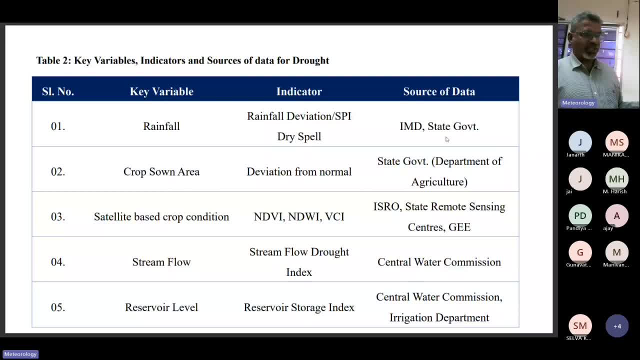 standardized precipitation indicator as an indices or the dry spell events. So for this we can use the IMB data, rated data Or the data collected in a point wise from various agro meteorological stations and all these things. Second one is crop zone area. that is, deviation from the normal. it is an indicator. 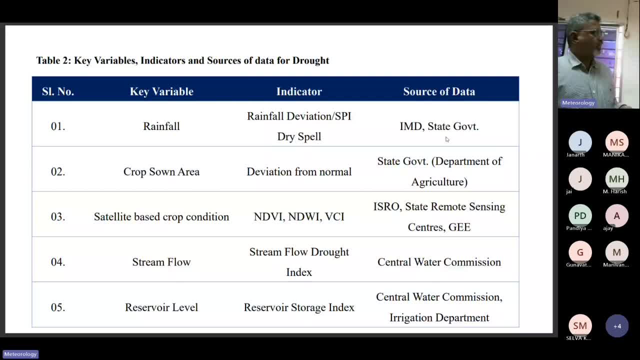 This is done by the state governments. Nowadays, remote sensing area, remote sensing indices or the products, are also being used to assess the crop zone area. So next one is satellite based crop conditions, that is, NDVI, NDWI and VCL. NDWI is nothing but normalized deviation in vegetation index. 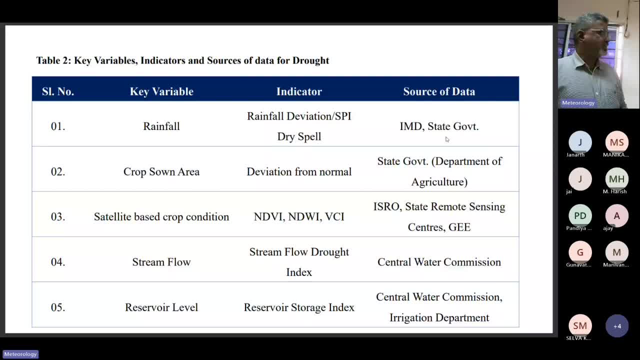 NDWI is normalized deviation in water index, that is, soil moisture index and VCI vegetation condition index And these are the products now available readily in Google Earth engine or ISRO or state remote sensing centers. They develop these products and readily made available. We need not to calculate all these things. 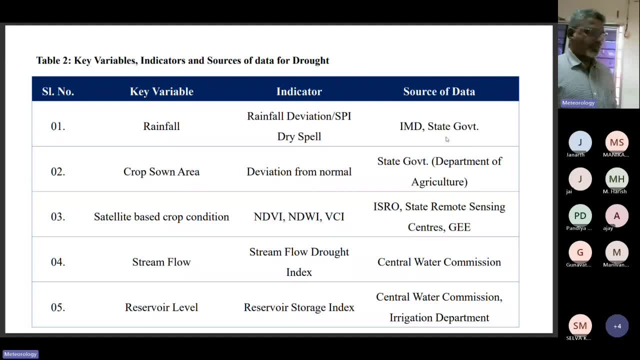 They are available readily. We can use it for monitoring the drought as well. Thank you, We are going to be monitoring the drought as well as the developing some drought mitigation factors. Coming to the stream flow, this is usually measured in the reservoirs stream flow or. 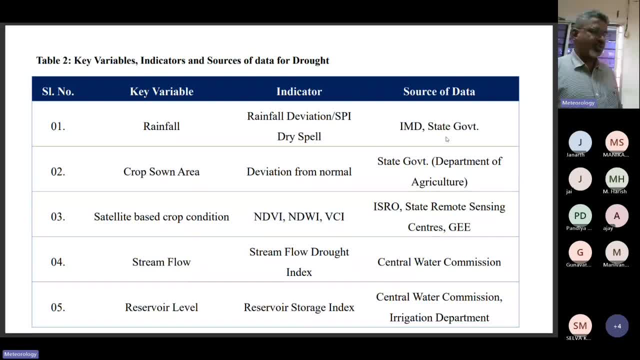 the drought index. Central Water Commission will give you this information And the reservoir levels may be Srivani Ram or may be Cauvery Dam, If the Central Water Commission or the recent development, they will be keeping the record of all those reservoirs and storage index. 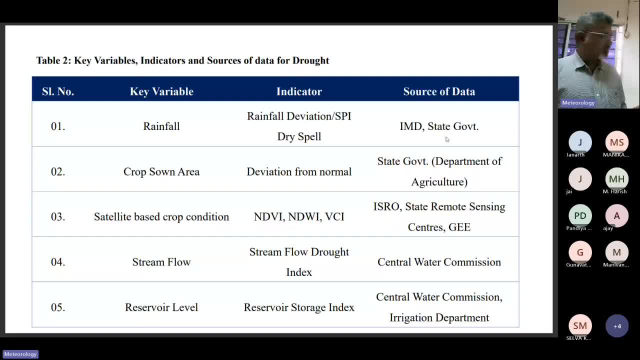 We can work out and definitely we can use that as an indicator for monitoring the drought figures. These are some of the indicators, or the parameters, or the measured observations, what we can use for calculating the drought indices. Coming to this, I already told you meteorological drought, soil moisture based drought, hydrological. 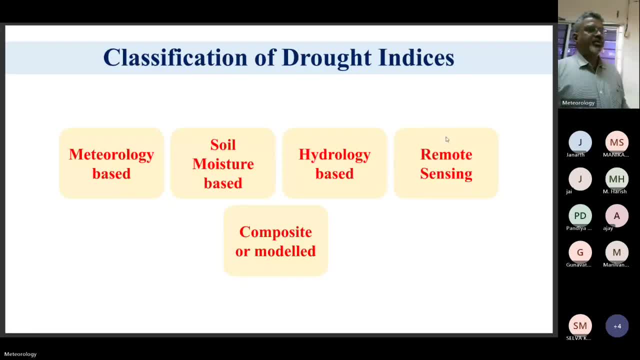 based drought, remote sensing based drought, and all these things can be combined. you can also have a composite or a modeled drought indices Coming to the meteorological-based drought indicators. it is very important that you have the OP system. So if you look at the overall might of the positive and negative, 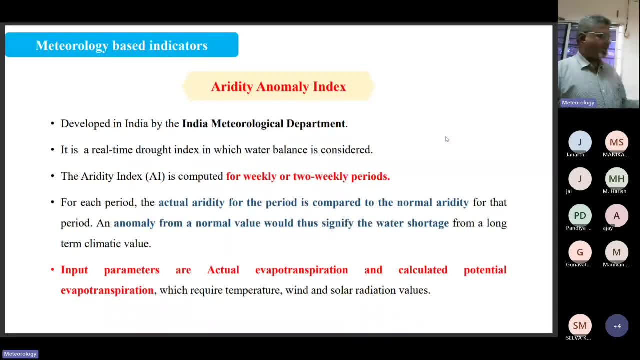 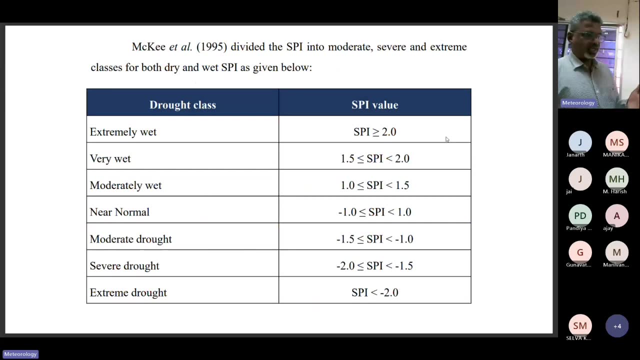 All of you may be knowing and you may be calculating all these things. I am not going to go in detail about these things. First one is Revitin-Armonky anomaly index, then SPI, standardized precipitation index. So based upon SPI, drought can also be classified into extremely wettable, extremely drought. 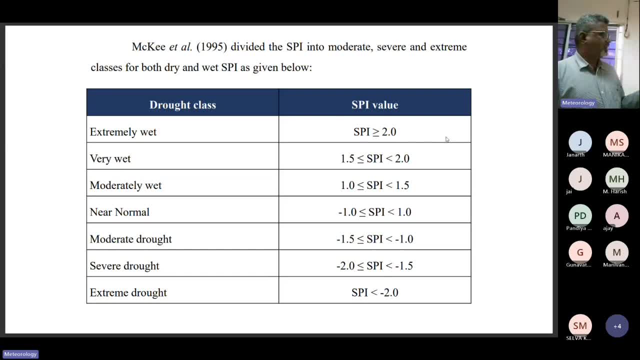 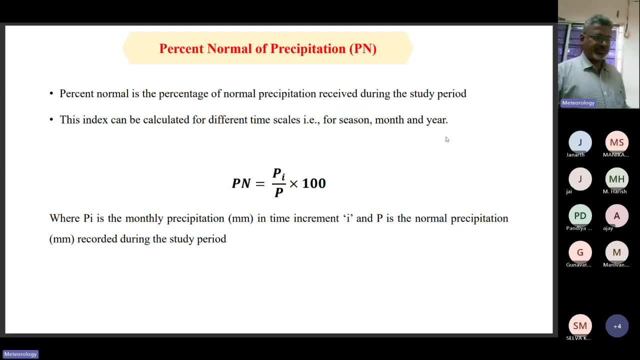 If the value of SPI is less than minus 2, it is extremely drought, extremely wettable is 2, as we have classified. Everybody may be very familiar with this. And percent normal precipitation is another one. how much normal precipitation, actual precipitation, deviates from normal? 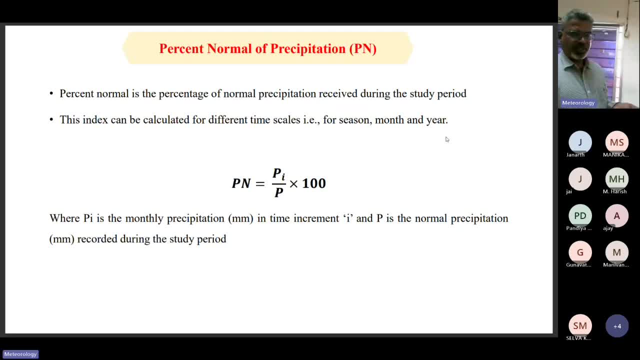 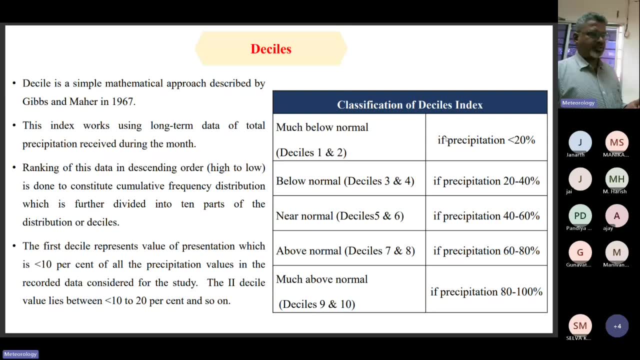 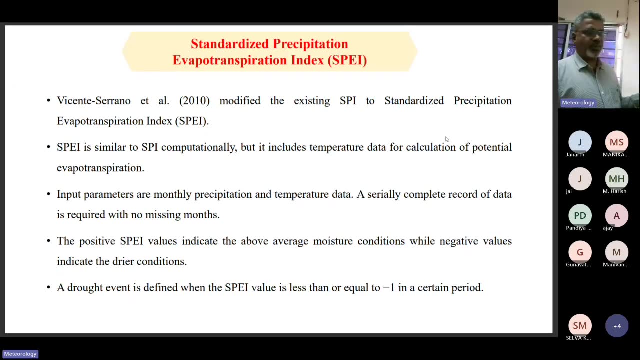 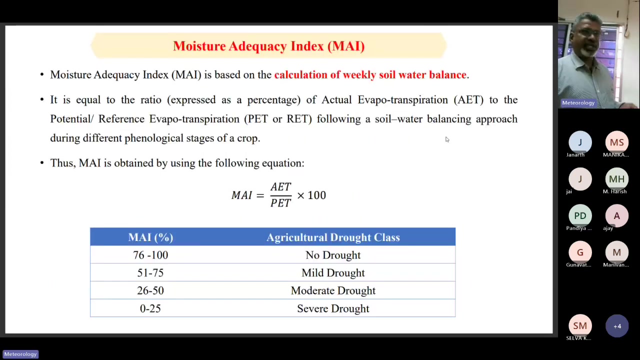 Another one is very, very Decaille index. this is percentage deviation once again. Then formal drought index, then standardized precipitation evapotranspiration index, SPI based upon only Wi-Fi SPEI based upon evapotranspiration, Then dry-spare index, then moisture adequacy index. that is AET by TET in contract. 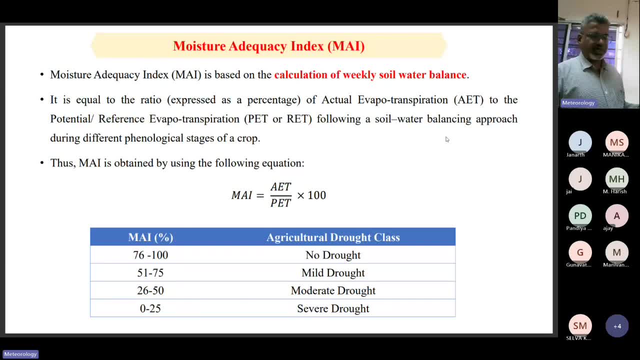 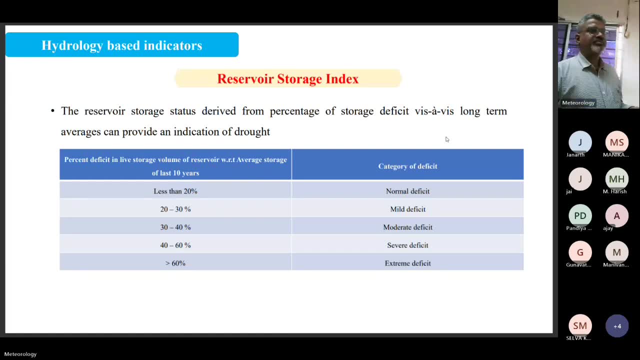 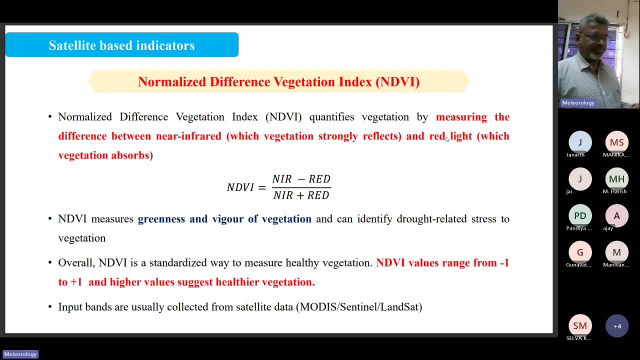 This also having classification called no drought, mild drought, moderate drought, severe drought, So reservoir storage index, depending upon the amount of water stored in the reservoir. Then this is some of the satellite separation indicators, like NDVI, normalized difference in education index. 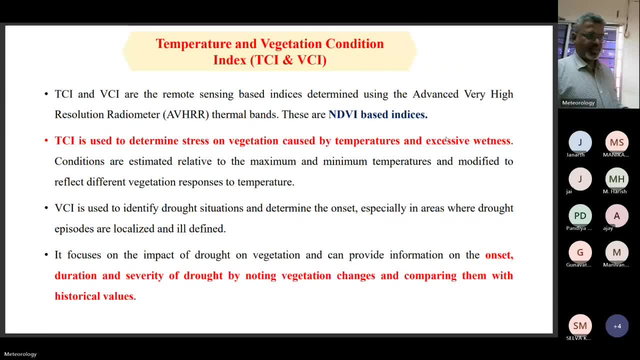 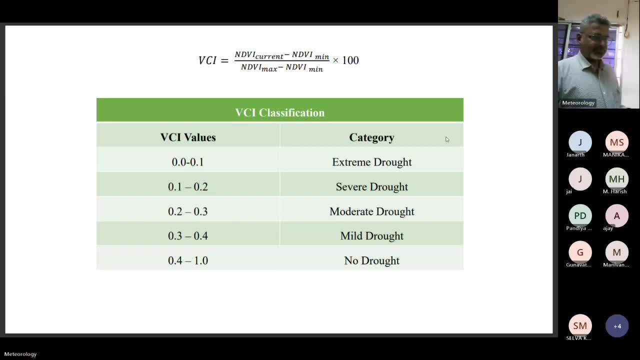 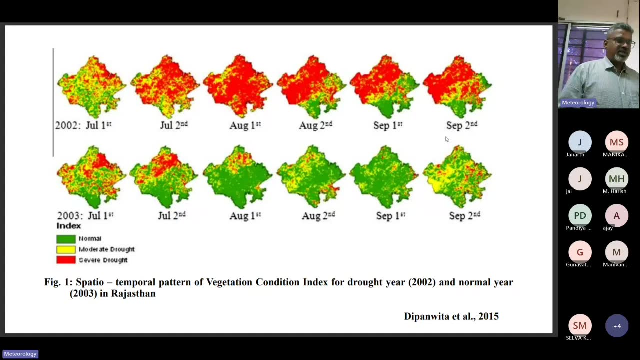 Temperature condition index and the VCI. So, based upon VCI also, you can classify extremely drought to the no drought, depending upon its value. So, based upon all these indicators, this is the first paper I have seen in 2015.. They have classified spatio-compatible pattern of vegetation conducts index for the drought. 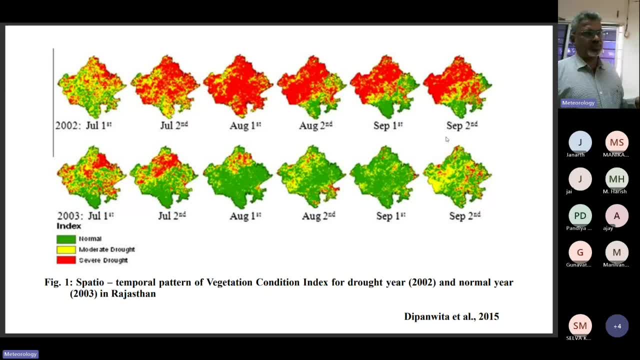 in the year 2002.. They have not taken 2002 because 2002 year is drought year. Yeah, Compared, they have compared with the 2003.. Whether this vegetation conduct condition index is good or bad, The vegetation condition index is going to towards the actual occurrence of the droughts. 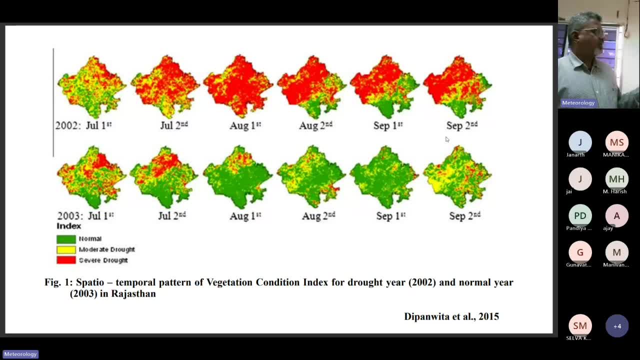 or not. You can see, wherever green areas are, that in the year 2003,, where the normal occurrence of rainfall has taken care, Say, for example, from July 2nd to August and September, most of the areas in Rajasthan are green. 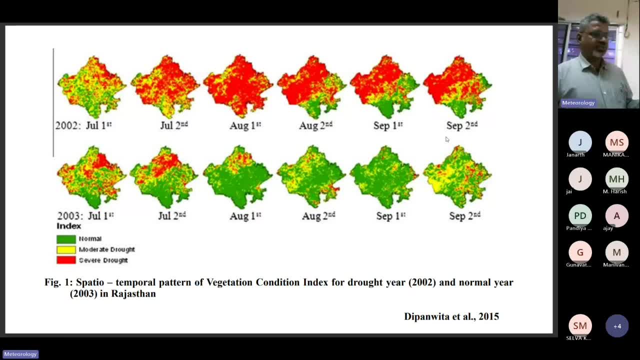 At the same time, during the drought year, that is, 2002, 2002, starting from July to August, after second week and September first week, most of the areas vegetation condition index indicates the clear occurrence of the drought That clearly indicates. vegetation condition index can also be used as a surrogator to 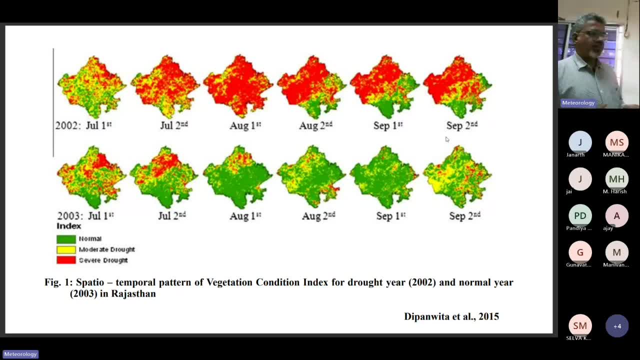 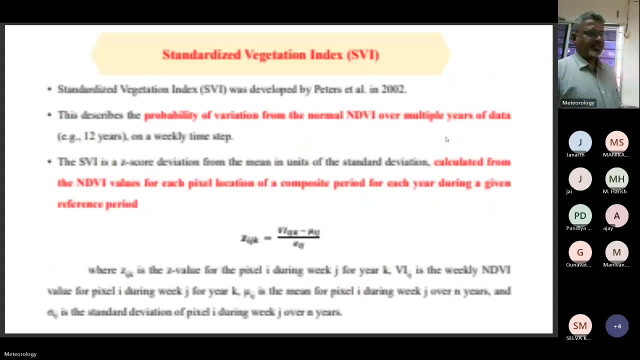 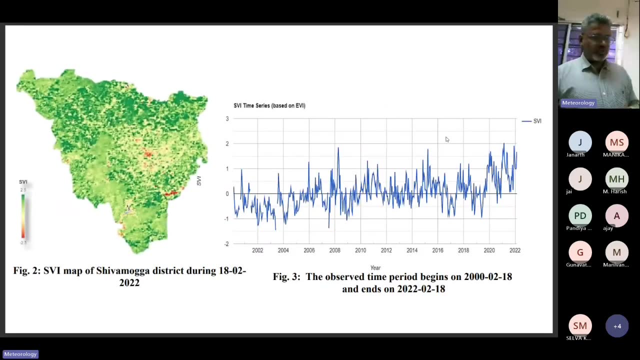 declare the occurrence of the drought as well as monitor the development of the droughts, Not only occurrence, development of the drought over a period of time can be done. Similarly, standardized vegetation index also. some of them I have used. See this, we have done it for by using Google Earth engineering for Sumaga. 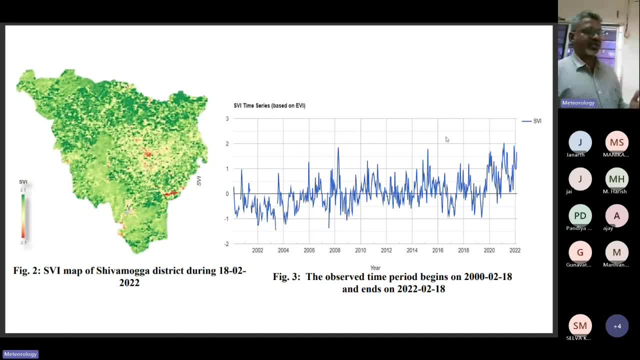 You can see starting from 2002.. Here your negative values are there. I think this animation is not working. here You can also see animation how it works and all those things, how the drought develops and all those things. So, starting from its soil, standardized vegetation index we can use. 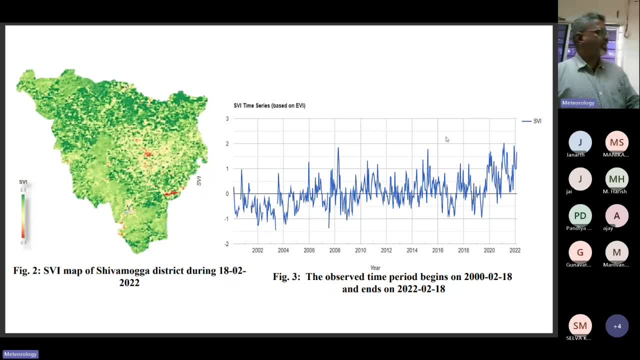 This is the Google Earth engineering products. We can see wherever these red areas are there. those are the areas where occurrence of the drought can be seen. You can see all these negative areas starting from 2002.. You can see negative is a monthly SDI. 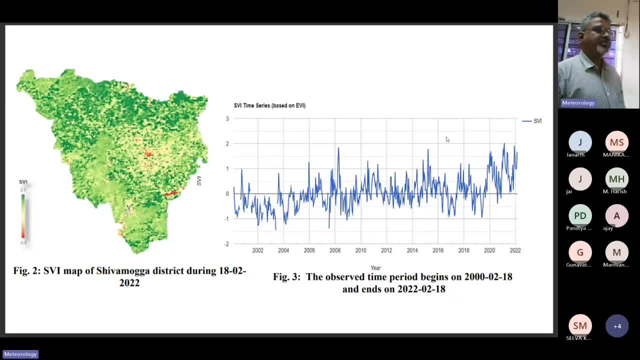 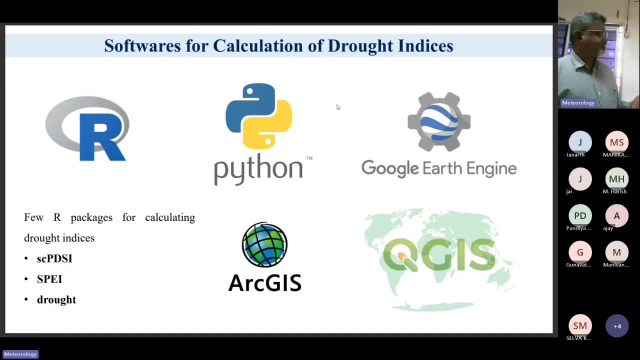 This can also be used in the year 2003.. This can also be used for as an indicator. Let me see How it can be used. Very recently, these indices can be class calculated by using programming tools like R, Python, Google Earth Engine, ArcGIS and QGIS. 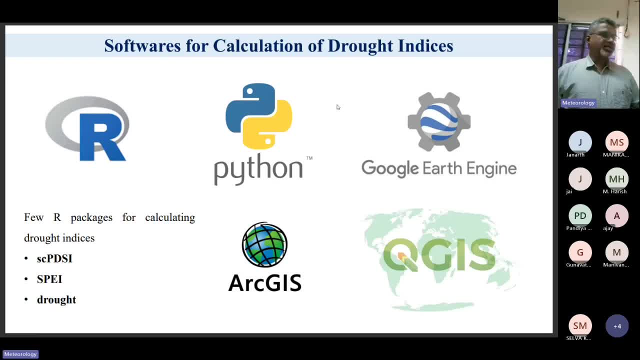 So the libraries available in R are SCPDSI- that is, the formal votes index- SPI- standardized vegetation operation index- and the drought. These are the some of the libraries or plugins. So if you have libraries or plugins available in R itself, you can invoke them and you can. 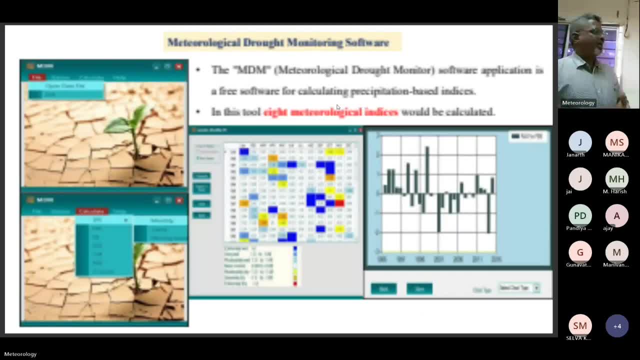 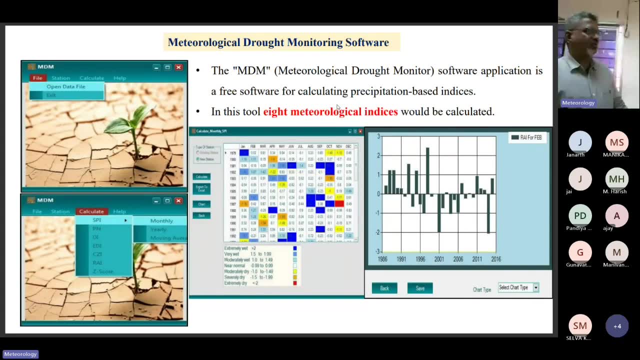 start calculating all these things very easily. Apart from this, you can also use one of the freely available software. most of you may be using drought monitoring software. There are two versions out there. One is paid version, another one is free. version is also there. 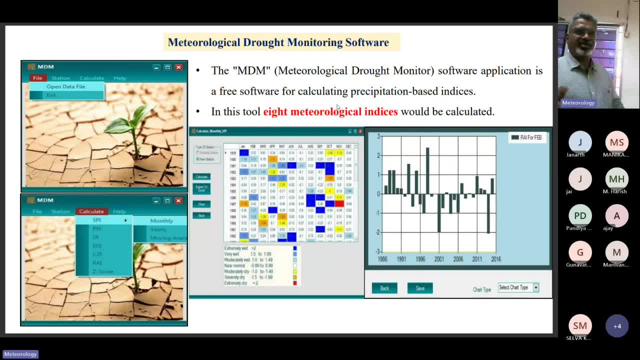 I am leaving my presentations here. You can take up your words and sit and see. So this presentation is available with your application. Thank you, This is the mythological drought monitoring software. this is developed by maybe someone in Iraq. this can be used very easily. 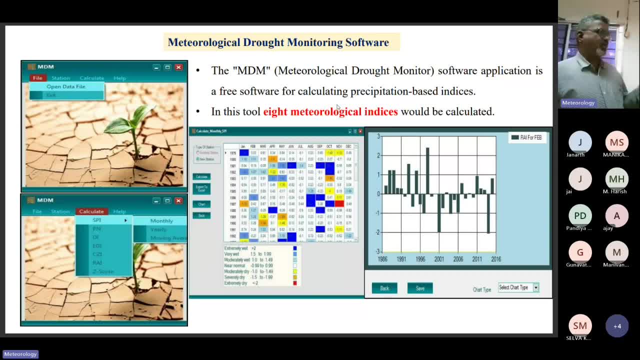 Just you do, whatever the parameters you have, If you have a moisture, a rain cloud, it is going to give you all the indices related to moisture. so, the rain cloud, If you have moisture in temperature in those areas, it gives you all the indexes based. 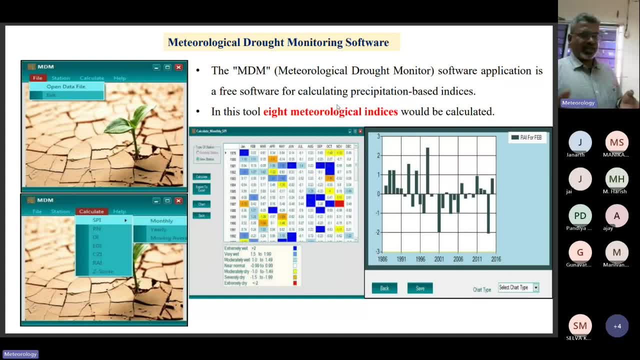 upon moisture as per moisture, So it is very easy to use moisture as well as rainfall. This is all the screenshots: how you can use and all those things So you can see here. another screenshot is the years you can see here, years you can. 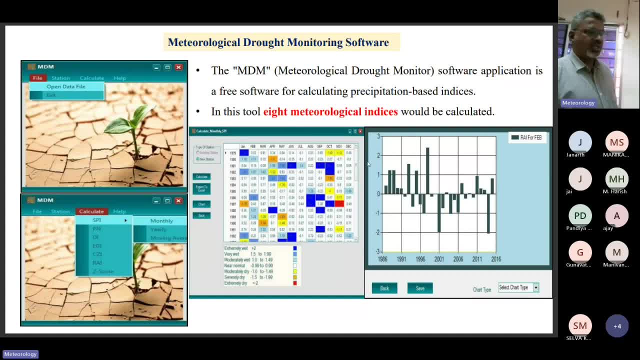 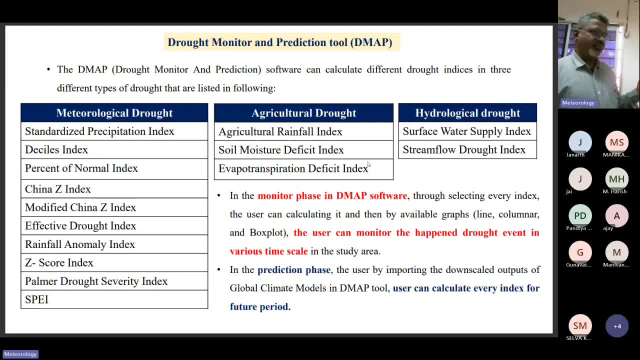 see the years. you can also see the months here and the occurrence of droughts and its specificity. So another one. what we have used is Drought Monitoring and Prediction Tool, DMAT. It is also available freely. If you contact the person in INI, I think they are going to give you this software freely. 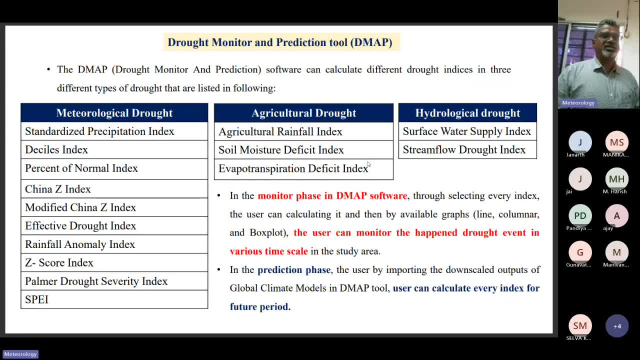 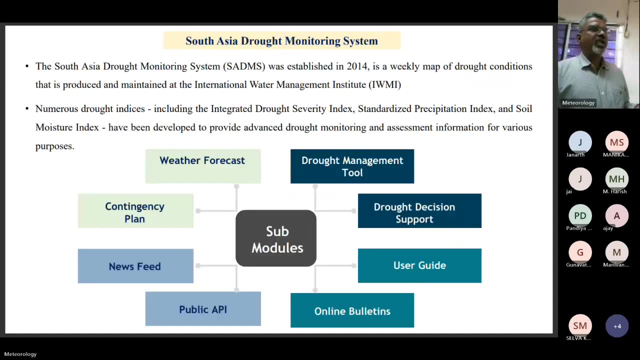 So you are also going to calculate meteorological drought indices, agricultural drought indices and hydrological drought indices- All these indices earlier used to calculate values in Excel. Now all these things can be calculated by a click of a button very easily. Then another one. I think Dr Koppilavani may be knowing this one. Dr Koppilavani may. 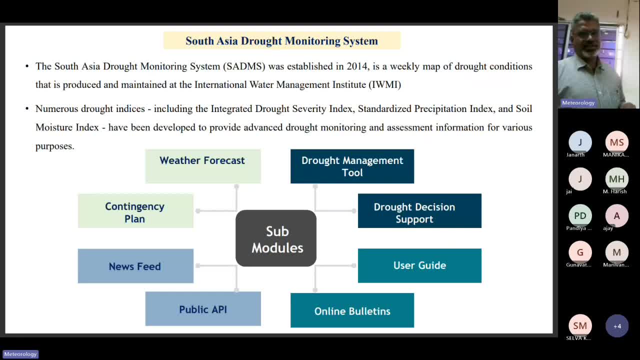 be knowing He may be attending the same training program about how you can use the SARAMs, That is, South Asia Drought Monitoring System developed by INI. It is also available on the net So this, also used for drought forecasting, can be done whether the drought is going to. 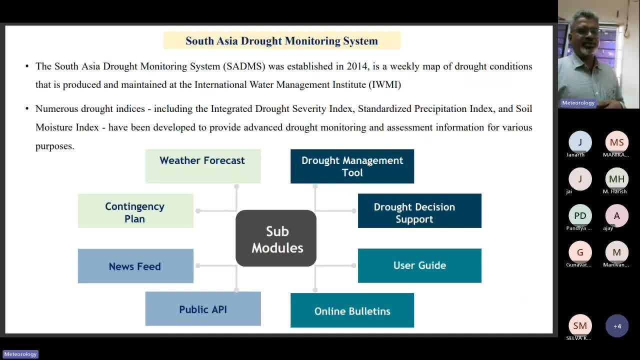 occur this year or not. Drought management tools are also available: Drought decision support system. If the particular month is experiencing this is the drought, what are the decisions a farmer can take? Those things are also there here and it is having the user guide public API news feeds. 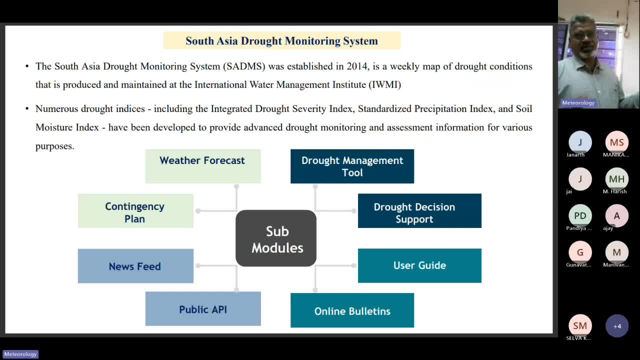 contingency plans, everything to have bundled into one software. It is an online software. you can use anytime to monitor it. Last year we used this to monitor the occurrence of drought over some of the districts and it is going to do some to an extent of 60 to 70% the occurrence of the drought that is. 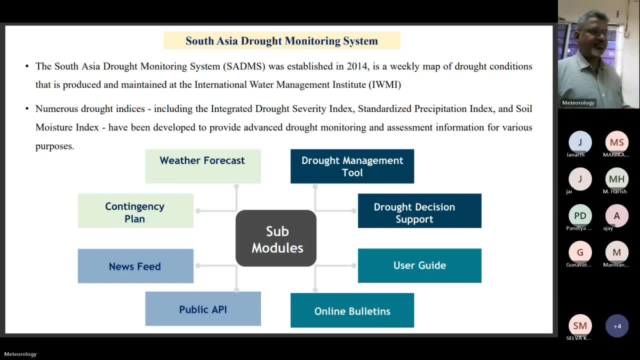 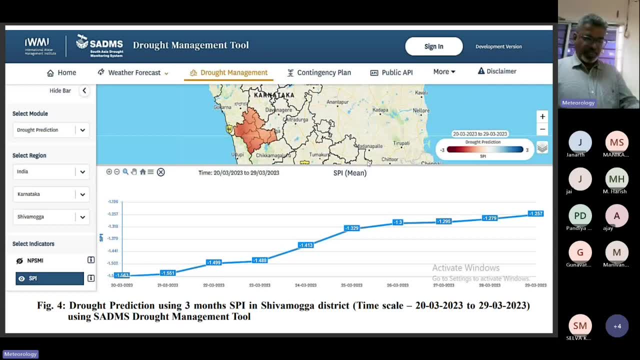 forecasting can be done very easily. This what we have done. This is some of the district, So how the drought has occurred, you can see here During the evening. During the year, just from 23 2013 to 23 to 29- 3, that is, March to March- we have seen 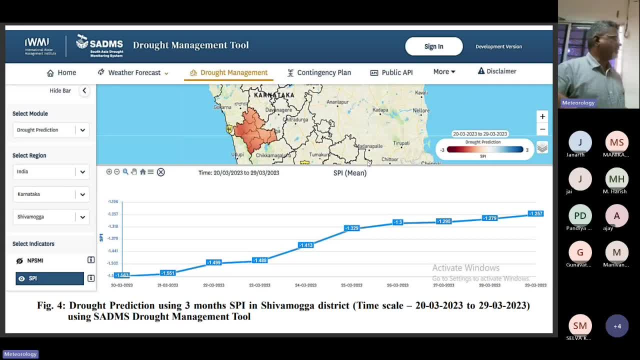 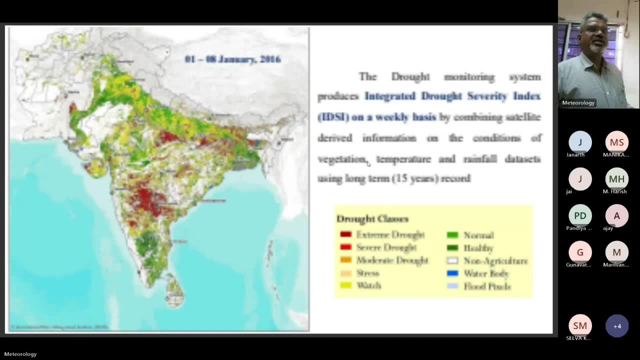 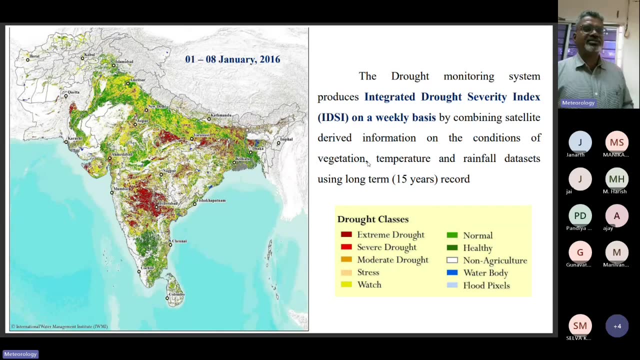 One month. you can see here the occurrence of the drought, how it is increasing. This also you can use very easily as a tool for drought forecasting. Apart from this, there is a drought management system. products are also available for India. Integrated drought severity index on weekly basis. 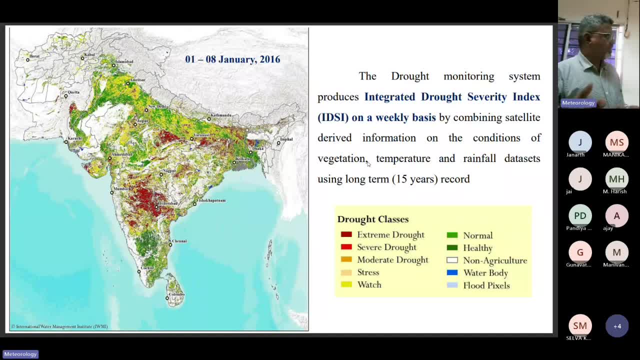 This can be done by maybe MNCFC as well as maybe in space application center. Both of them will also be used. This can also be combined with our agro advisories so that we can know whether the drought is going to occur or not going to occur. 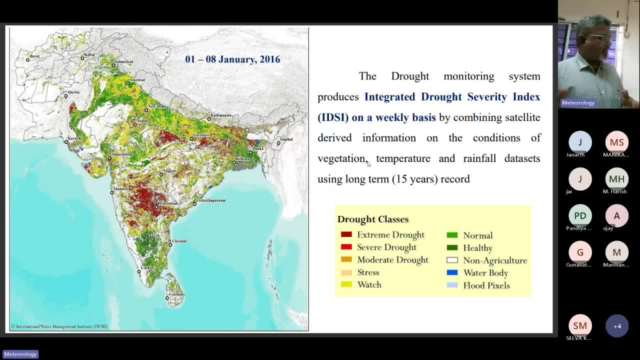 If the drought is occurring very frequently, then what are the mitigation options? or can we tell the farmers to postpone the showings, or whether can we advocate a farmer to take a loan? There are so many different things available and we can give you all those advice on the 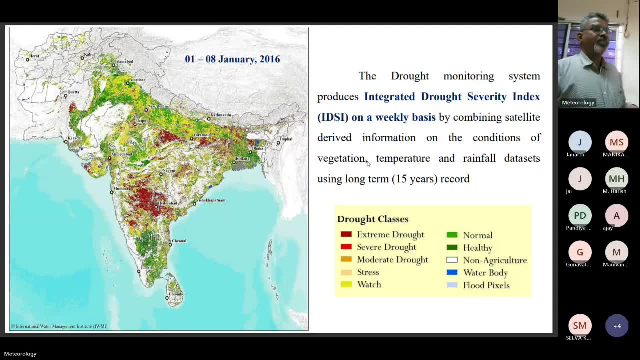 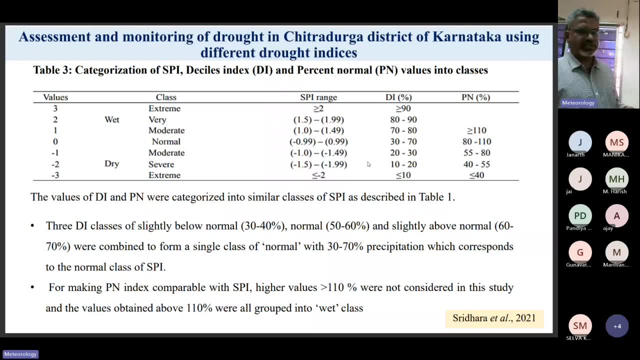 integrated drought severity index on weekly basis. So we have used same SPI- the drought index, as well as percent normal index over drought heat district, that is Chitraurga district, which is very largest rainfall receiving district in Karnataka, And we have published this paper in Zerlapagra meteorology. 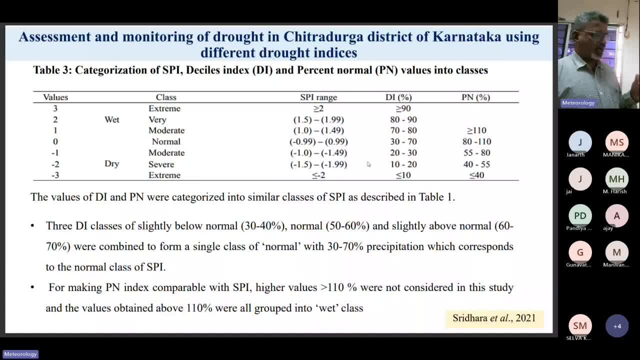 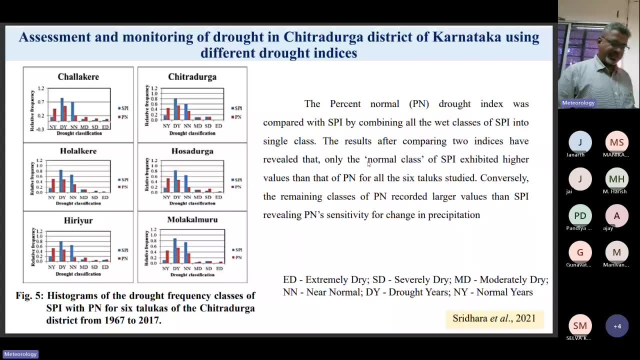 And we have taken at least 1.5 million units of rainfall per day And we have also done how we can monitor the occurrence of the drought on various talakas, that is, the hovelies coming in that, And we have also given some recommendation to the administrators. these are the talakas. 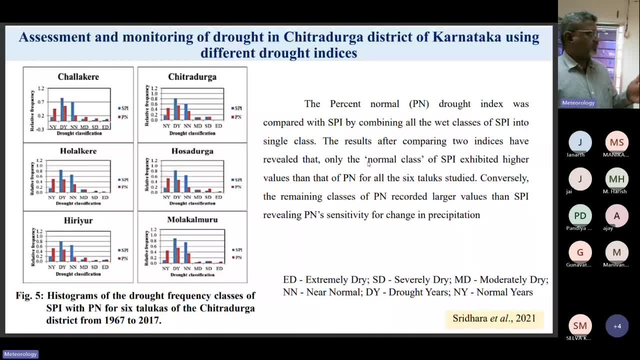 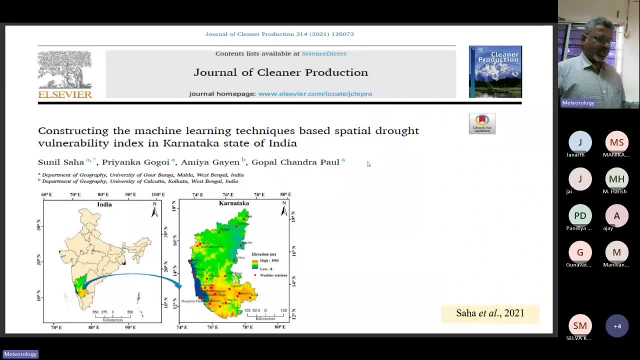 where occurrence of the drought will be very frequent, so that every year we would have some contingency plans like that, similar to that that one So very recently. all these things, that is, that meteorological drought, hydrological drought and socio-economic drought can be combined together and straight together, and 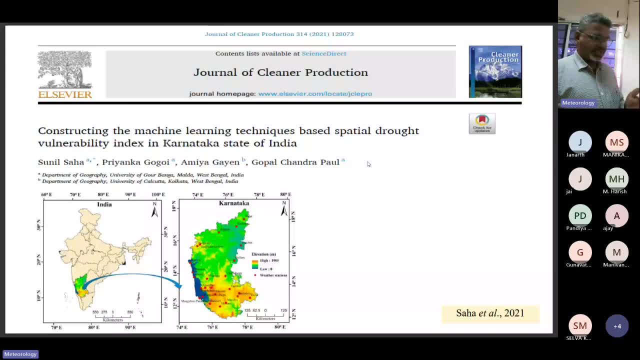 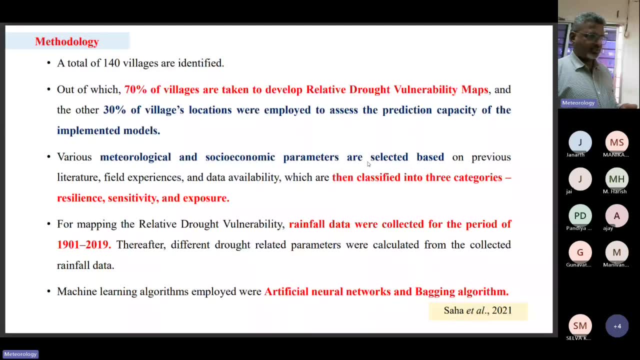 can be developed as of the drought, vulnerable areas and mitigation options, By person Sunil Saha. he worked very closely with us and he developed a map like this. So he has taken all the socio-economic data, demographic data, all those things he has. 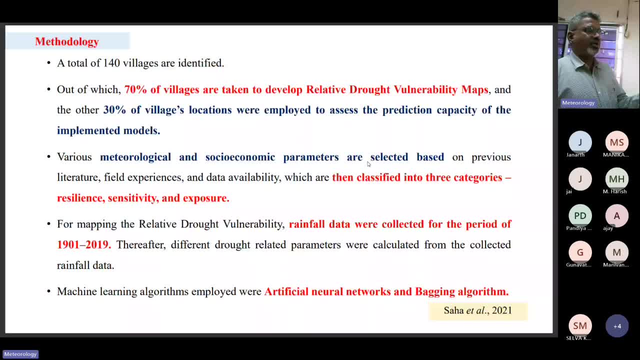 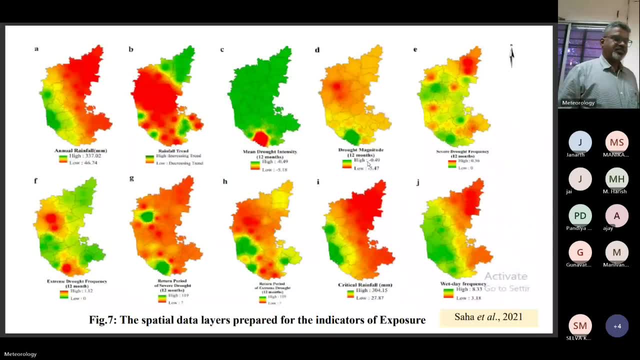 taken. So like annual rainfall, rainfall trend, mean drought intensity. so many things he has taken, So he has taken all these things into consideration. Then we have: he has mapped the spatial data layers prepared for the indicators of exposure. How many areas are exposed to drought? 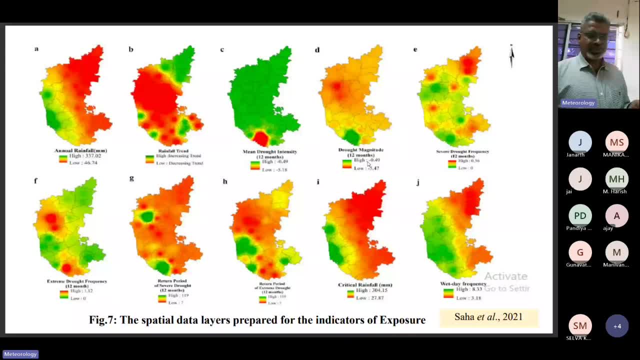 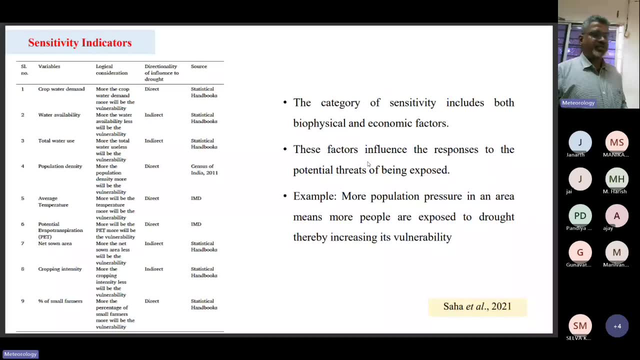 That is very important. Exposure is how many areas are exposed to the drought. So, based upon this, he has taken crop water demand, water availability, all those things. Then he also done the sensitivity. Once the exposure, which are all the districts, are become very, very sensitive to you this. 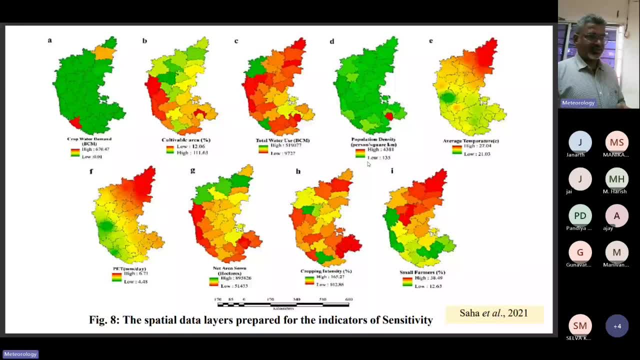 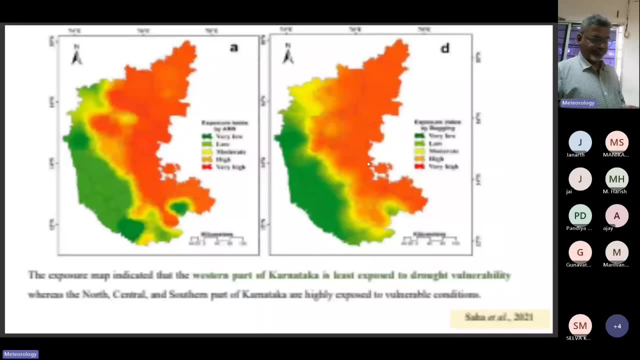 can also be done: Exposure Sensitivity, Sensitivity and resilient indicators. So which are all the districts where the mitigation options are very much needed to make that the drought occurrence is going to be reduced? the impacts of the drought is going to be? 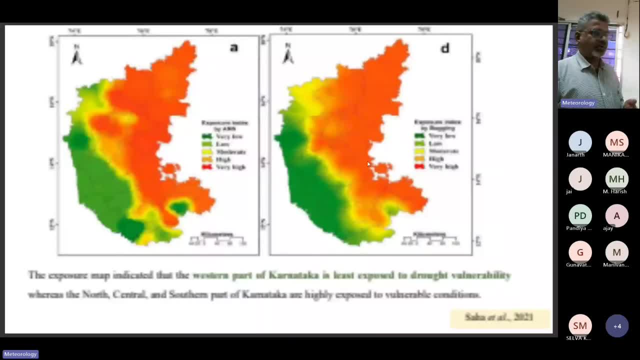 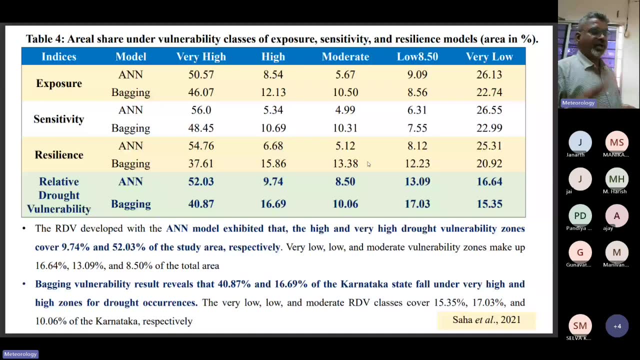 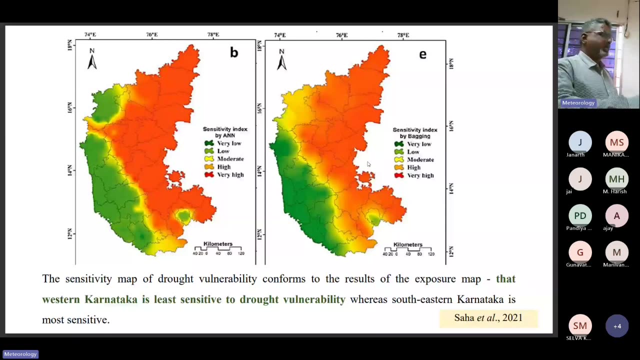 reduced. They have also used machine learning algorithms like artificial neural network bagging, then so many things, And they also classified the exposure as well as the severity and sensitivity indexes, and they clearly told that the most of the coastal areas in Karnataka are very less sensitive. 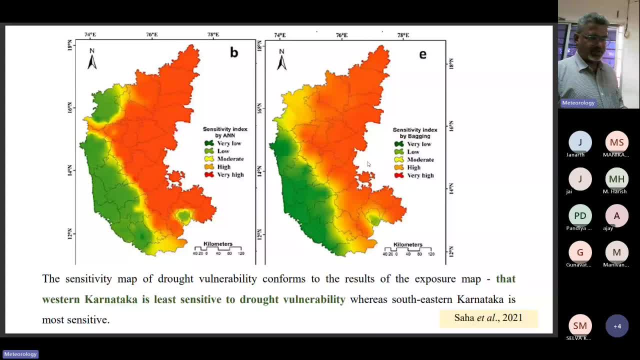 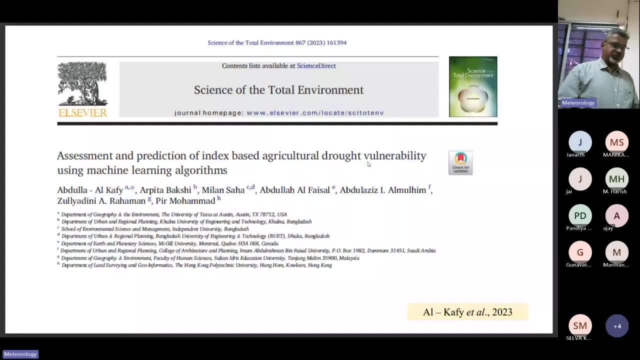 to the drought and most of the northern Karnataka is highly sensitive to the drought. So very recently- this is very, very important- Most of the advanced tools one person in Bangladesh, Al-Khafi he, has used: assessment and prediction of index-basis drought, agricultural drought vulnerability using machine learning algorithms. 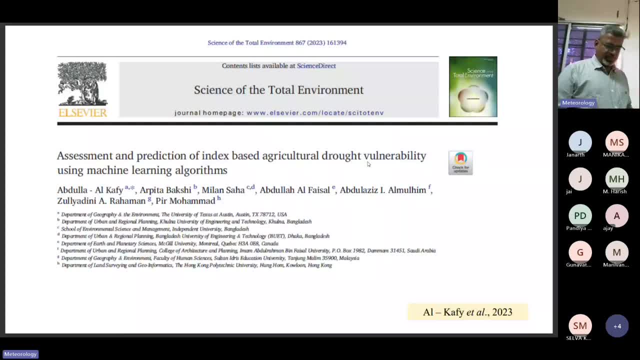 So, whatever the work Saha has done, most advanced stage this person has used Now he is a PhD student in Texas University in the Department of Geography, So he is a very good person. Most of them who are working in agro-metrology, especially on drought, refer the work done. 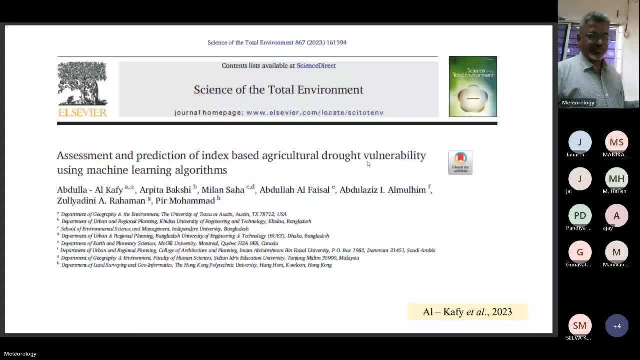 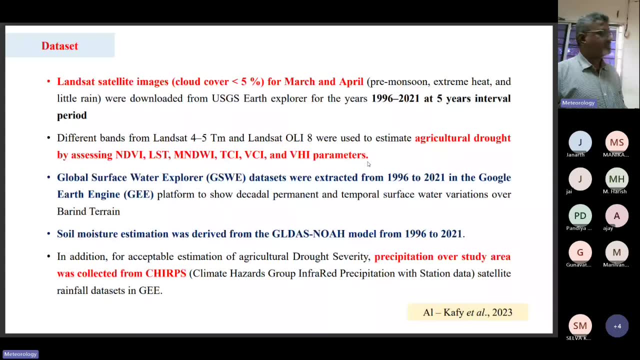 by him. He has done most of the work by using only Google Earth engines. No other things he has used. You can see for the Bangladesh he has done. This is the workflow how he has used. He has taken the satellite imageries. 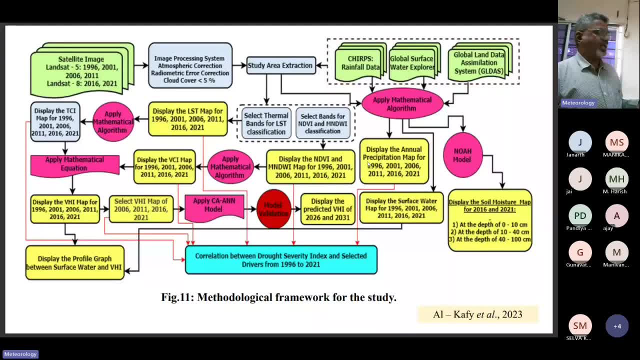 He has done image processing, study, area extraction. Then he has used all the freely available precipitation products, like Global Surface Work Explorer, CHRIPS, Global Land Day Assimilation Data, All those things he has assimilated, starting from, starting from, temperature convection. 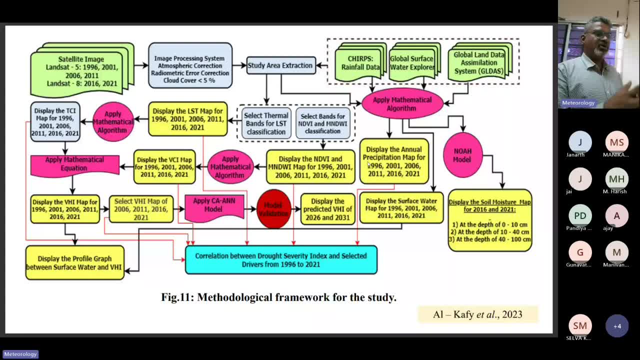 index, then land surface temperature index, All those things he has taken into consideration And he has correlated the drought severity index. So earlier we started telling about the drought based upon only rainfall, its deficiency. Now so many things can be combined together just to tell how does the drought can be severe. 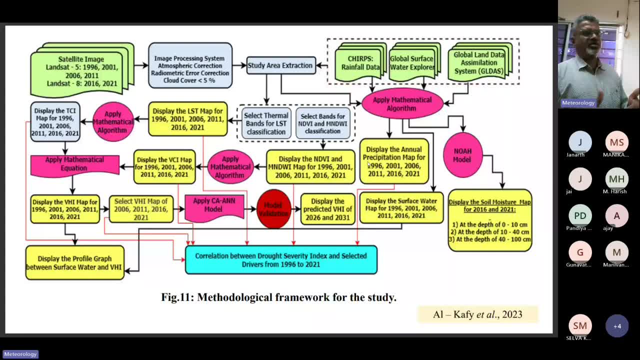 It takes everything into consideration: Hydrological drought, geological drought, socio-economic drought, soil condition index, temperature condition index, canopy condition, index, crop growth. various other endeavor can be combined together. So, based upon this, only NDVI, TCA and VCA. 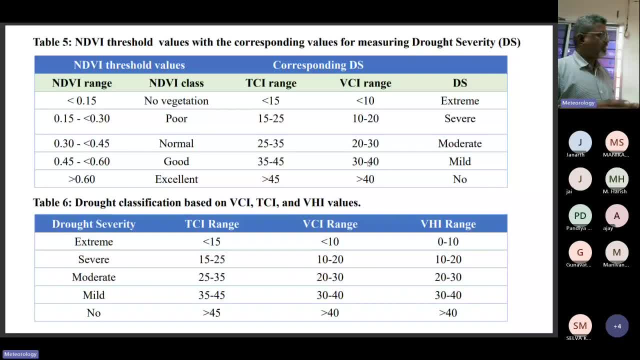 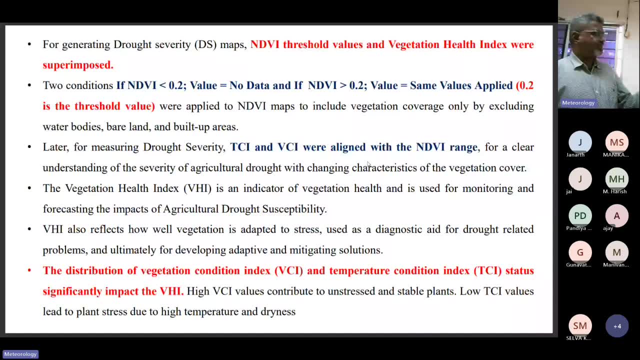 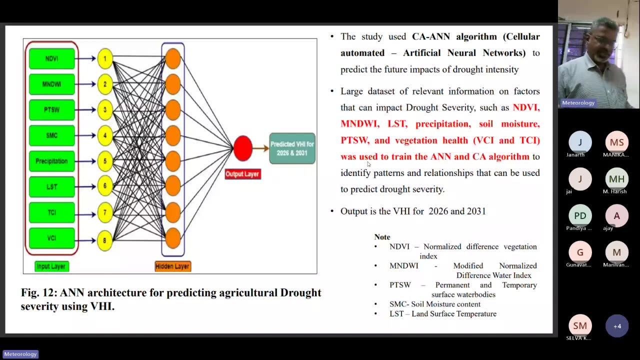 So they have classified them into extreme, severe, moderate and further. they have used these things to map the severity Once again. they have used all these artificial neural networks and all these things, NDVI, all these things They have stated one above the other to get the drought severity index. 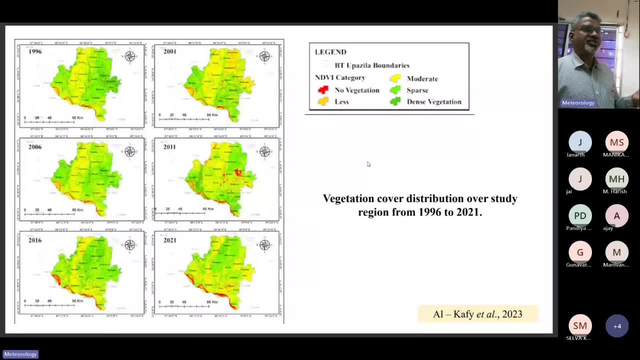 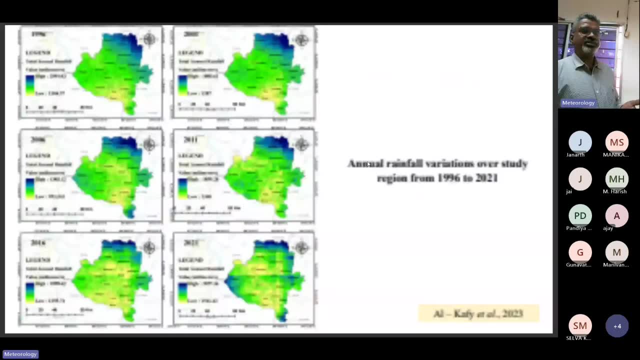 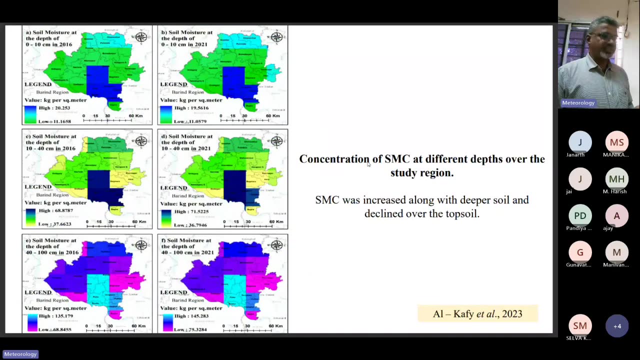 This is what the drought severity index. So no vegetation, less vegetation, moderate vegetation, sparse vegetation and dense vegetation. Then one is annual rainfall variations, Then concentration of SNC, soil moisture deficiency, soil moisture concentration, Then land surface temperature in degree Celsius. 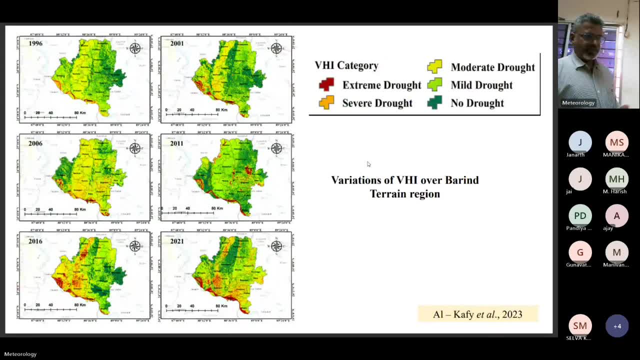 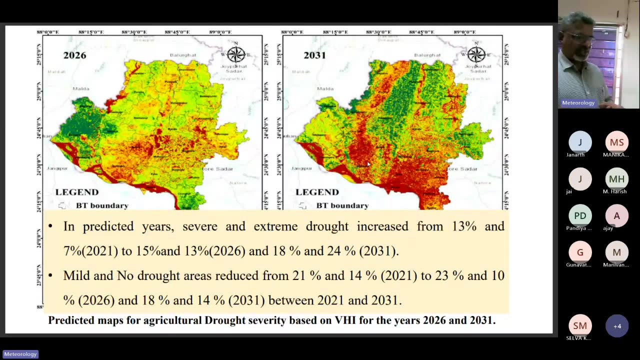 Then vegetation condition index, Then vegetation hierarchical category, that is, vegetation condition index- where it is going to be less, where it is going to be high or moderate drought or severe drought can be done. And finally they have predicted the occurrence of the drought- extreme drought- in the year. 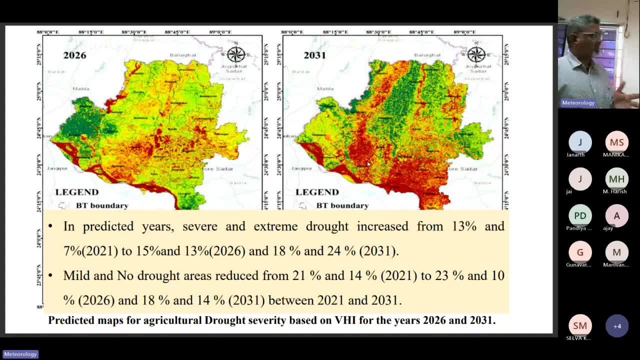 2041,, 2026, and 2031.. We have future climate data also. They have infused it for forecasting the occurrence of drought in the next years. This is the most advanced data one can refer for monitoring the drought. So they have used. 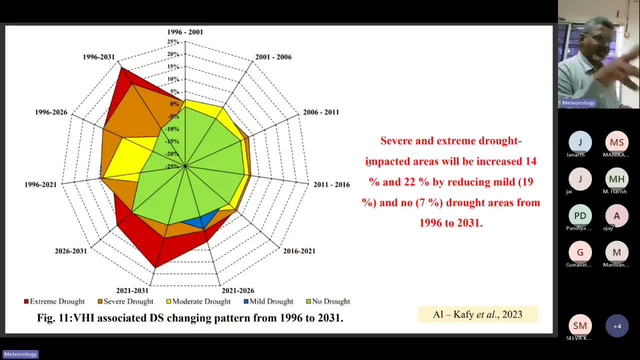 Everybody may be knowing, This is Umbrava diagram Everyone uses nowadays. Severe and extreme drought in tax areas, they told very clearly, will be increased by 14 percent and 22 percent and reduced by 19 percent, And there will be no droughts in the areas from 1990 to 60, 2010,. only 7 percent. 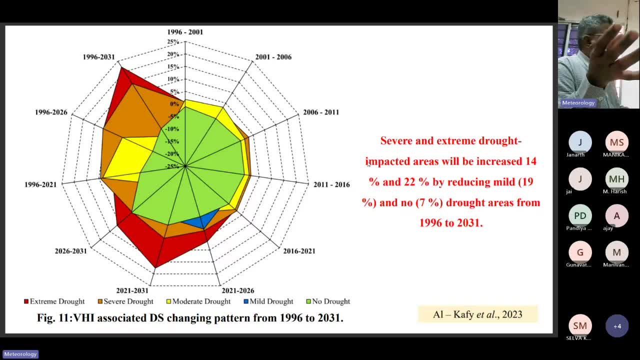 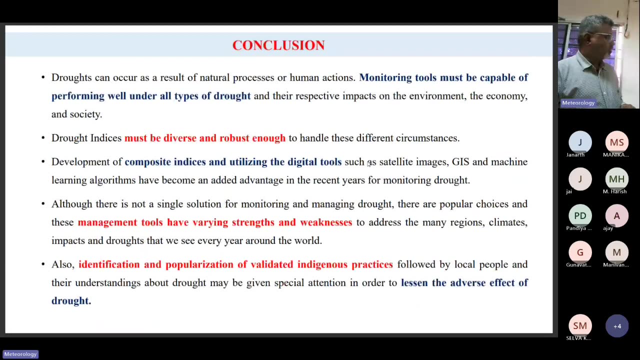 This percentage of area will be affected by severe drought to the moderate drought or the moderate drought, based upon PHI and the data. So so far, I have taken some time to tell you about the drought indices, software algorithms that we can use, all the software that we can use for monitoring drought, starting from 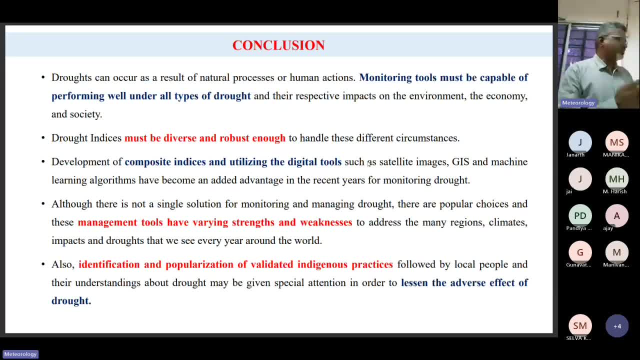 beginning calculation of just rainfall degrees and how we can combine most of the conditions with drought forecasting and all those things. So I thank you very much. I thank you very much for Dr Satyamurthy, as well as the Coming Agriculture University. 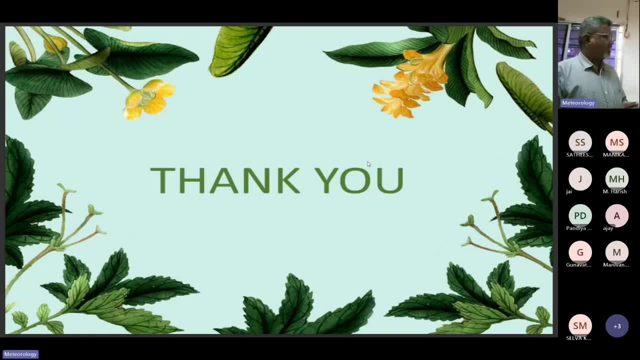 for giving me this opportunity to say a few words about monitoring of the drought. If you have any questions, we will have some time for some more sessions. If you want any of these things, the presentation will be here. You can take, You can subscribe. 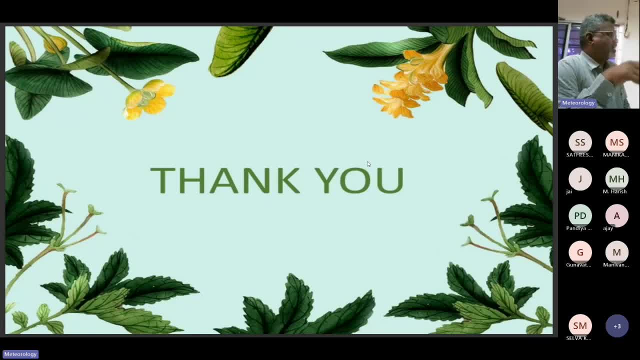 So last time when we came here, we gave something about how we can use these algorithms for forecasting the yields and values. Thank you, Thank you, Dr Satyamurthy. So let's get back to Whatever things I told you as invite. some may ask and ask that. 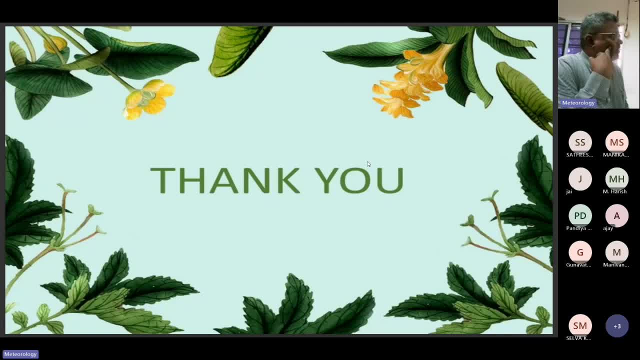 And I got some pieces from Dr Satyamurthy's athecial department on about drought-severe industry, drought intensity, SPSPS, all those Right On those. in the future scenarios, as we have done, We can actually help these things and 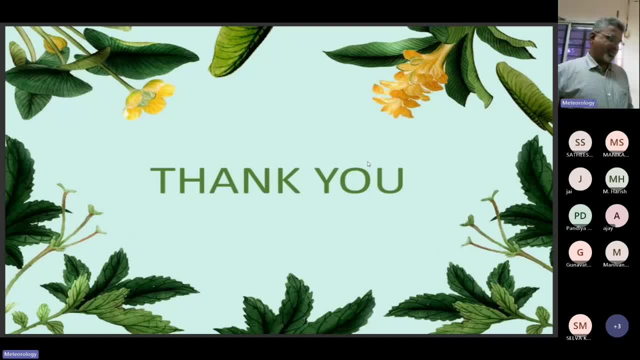 All the support's out there. Wow, We can improve all the data right. Most of the softwares are in fact. I learned from your CA department, in fact, because I am coming here since 1998.. Thank you, sir, for the informative and very useful presentation. 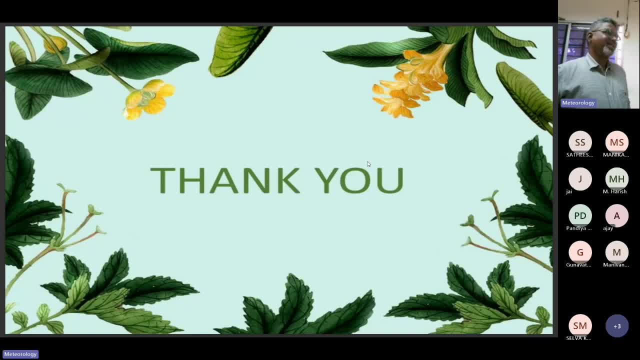 As a plant biology student, I am a non-pharmacologist and you are a great person. to clarify the answer to this question, Is that the question? Yes, sir, I have a very good understanding of the product and technology available in the market. 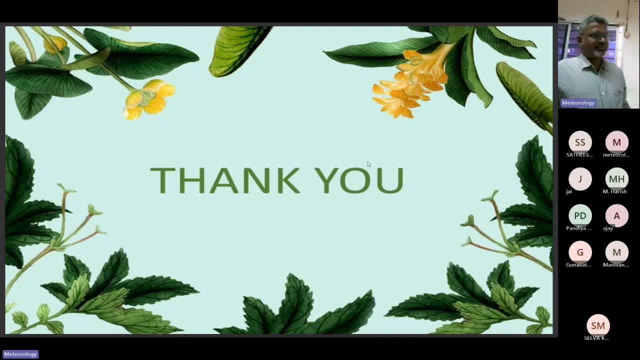 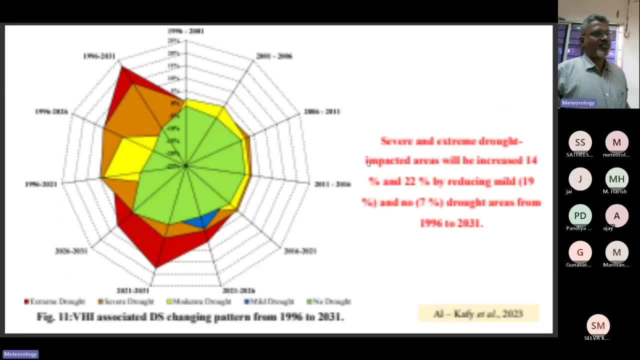 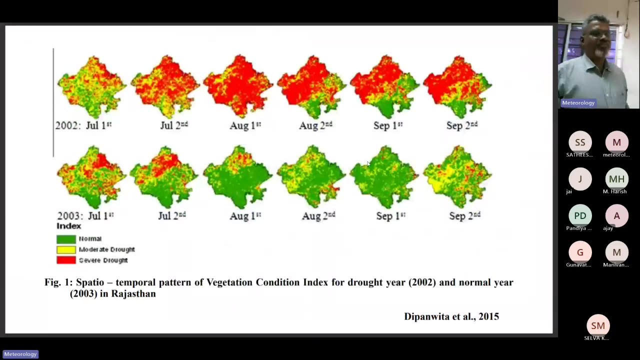 The highly efficient software available in them is tremendous. Yes, From what I know, the international market is very well known, so this is a good thing. The highly efficient software is not very efficient. it is really very efficient. I have to say that we have a very good product market. 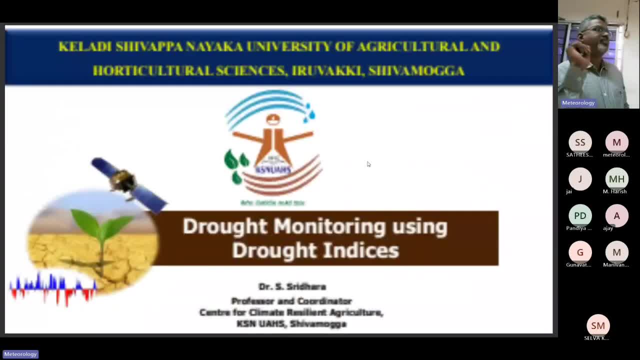 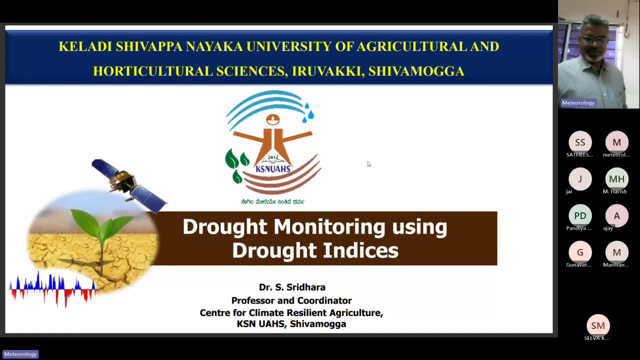 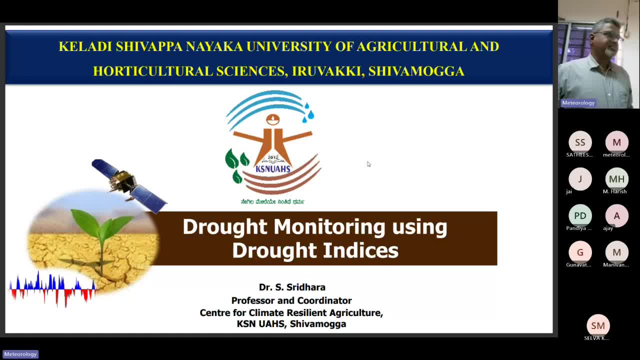 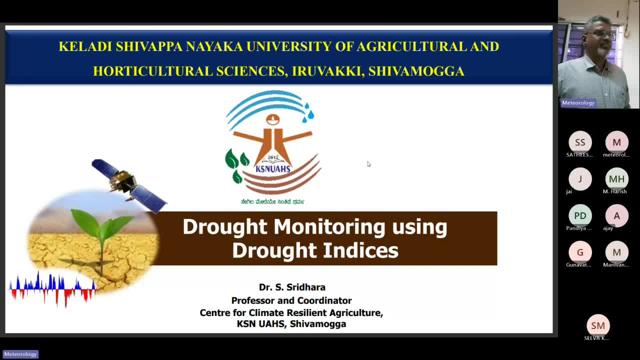 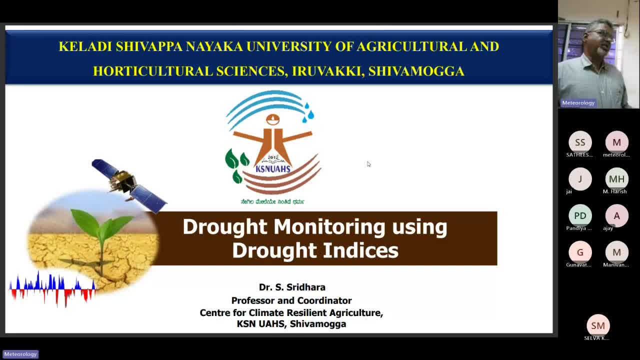 Thus, sozusagen, Whenever the temperature increases, day temperatures are going to increase- we are going to trigger the occurrence of the drought. depending upon the efficiency that I have found in the previous weeks, That is going to definitely trigger the population growth of all those whiteflies, as well as. 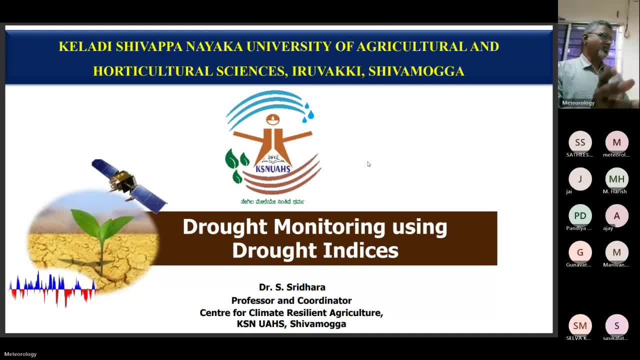 the creeps. Those are the main vectors for the occurrence of these virus diseases. So in fact, we have a record for the past five years. how does the increasing temperature increases the population of these creeps, as well as the whiteflies, their morphology? 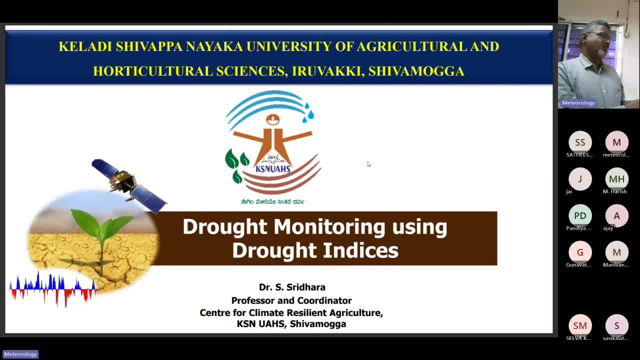 their fecundity levels will increase and how do they transmit these virus diseases? Definitely, this is a precursor. So that is our approach to virus diseases, how to describe them. Now, coming to the occurrence of the drought, and especially rain.